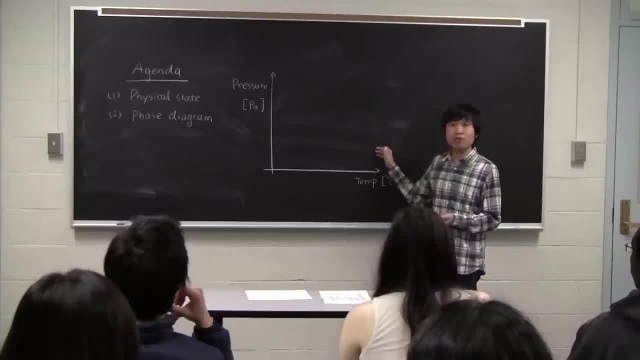 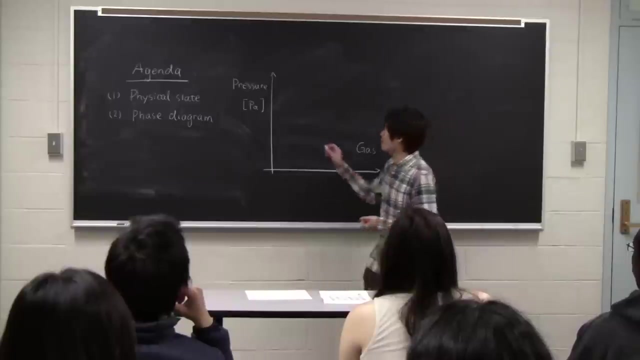 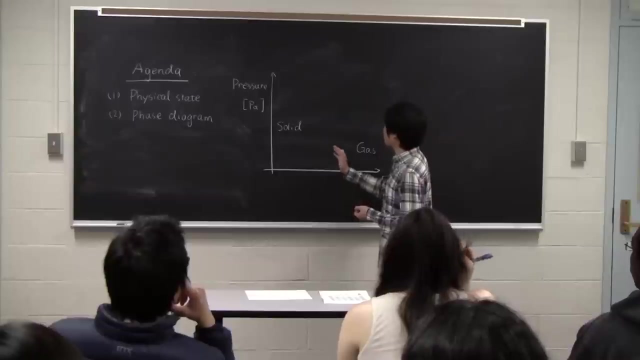 this is the high temperature space. Low pressure water will exist as Correct, Correct, So this is the gas state. And at low temperature, high pressure water will exist as Solid, Solid, Great, And at moderate temperature and pressure, water will exist as liquid. 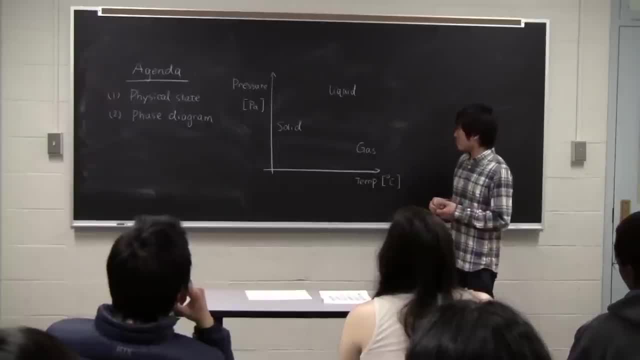 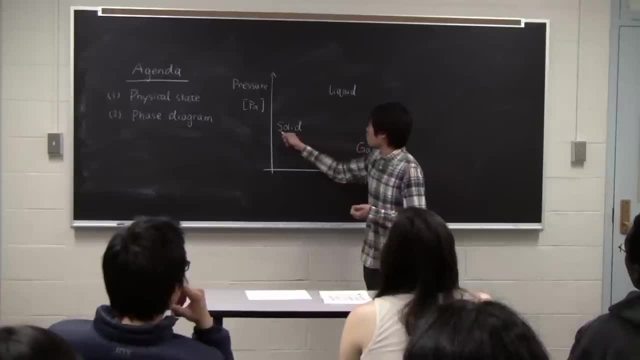 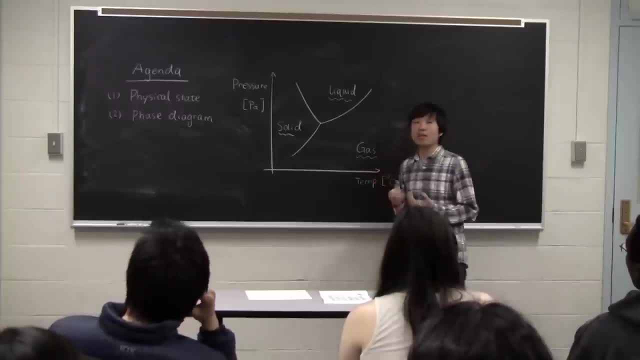 condition that a that two phases can coexist. So for example, at 100 Celsius, the reaction in one state, the reaction in the one state, the reaction in the other state, the reaction in the other state, the reaction in the other state, the reaction in both states are the. 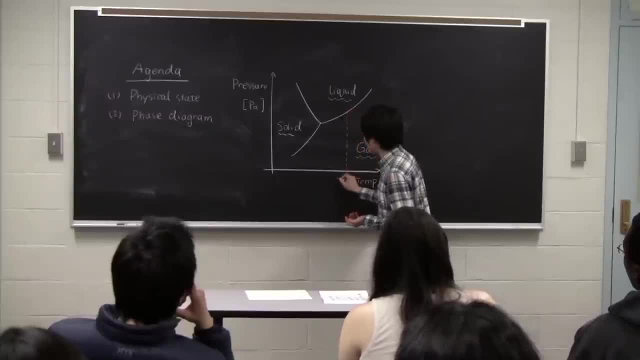 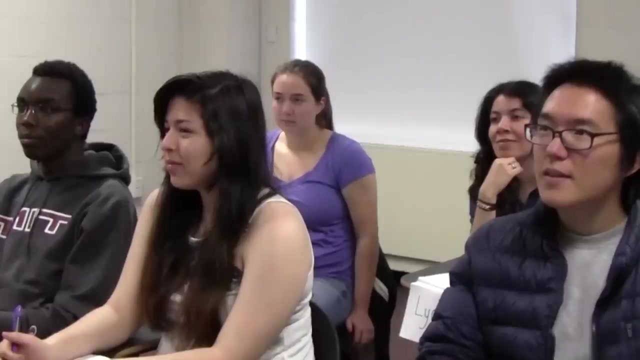 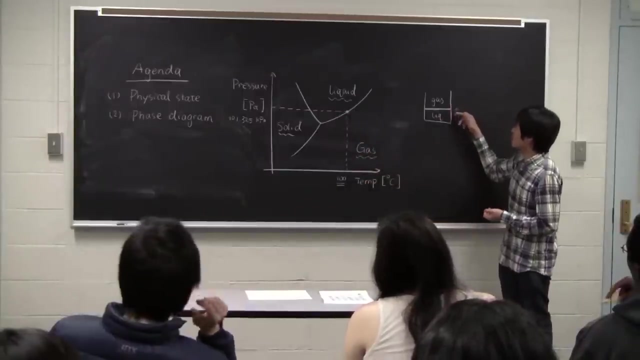 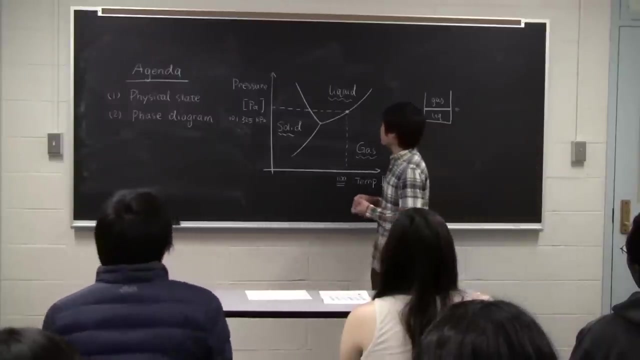 same, Okay, 100 Celsius and 101.325 kPa. So at this specific pressure and temperature, water can exist as gas and liquid simultaneously. So far, so clear, Okay, and there's an intersecting point of these three lines. 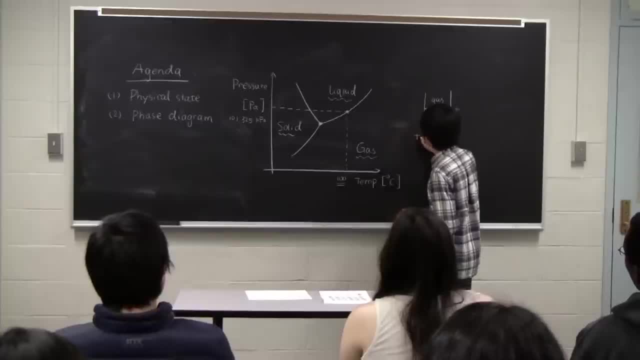 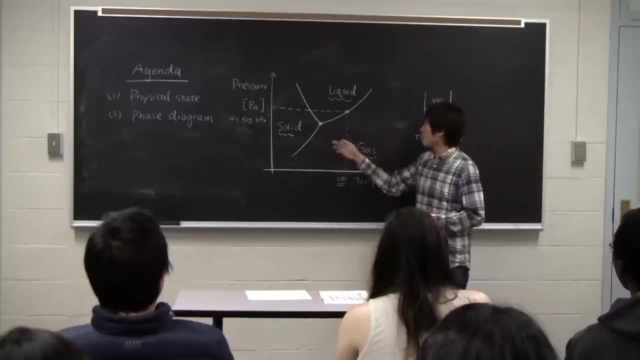 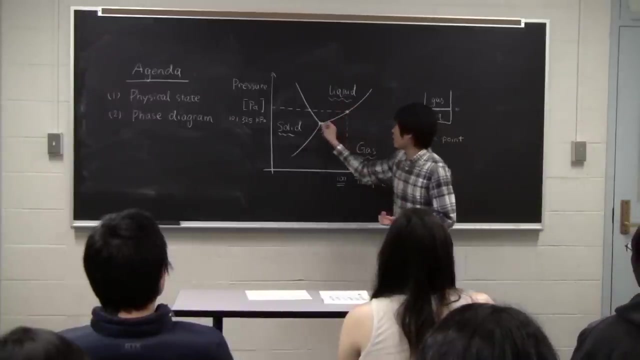 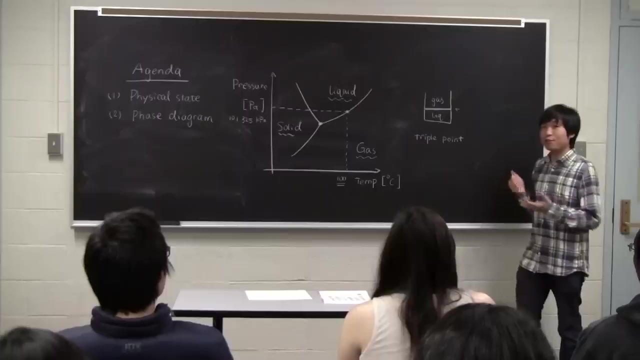 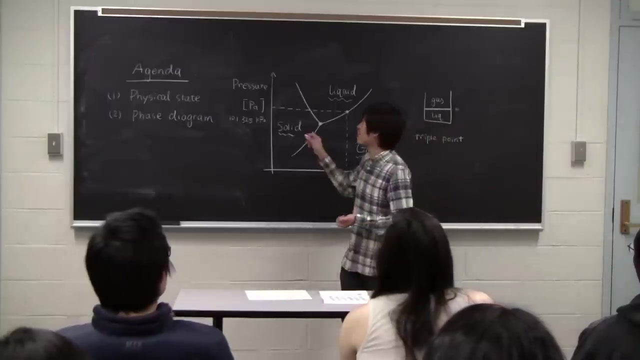 This intersecting point is called a triple point. At this triple point we have three phases coexist, So liquid, solid liquid and gas can exist at this specific pressure and temperature. Okay, so now there's a question. Supposedly you're on the mountain of Himalaya and then you know the pressure is slightly. 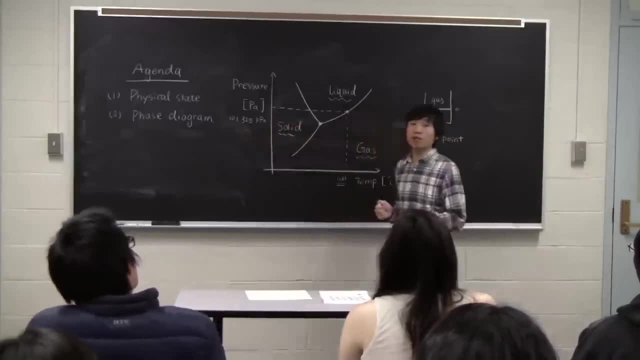 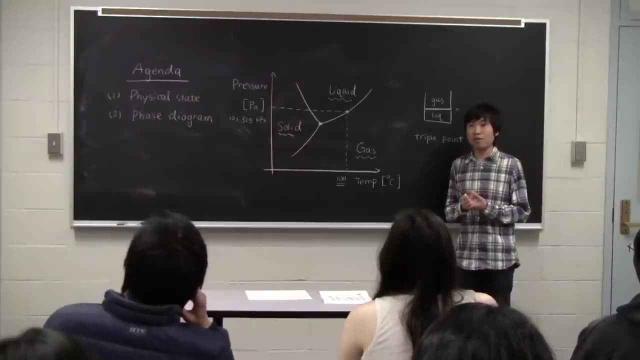 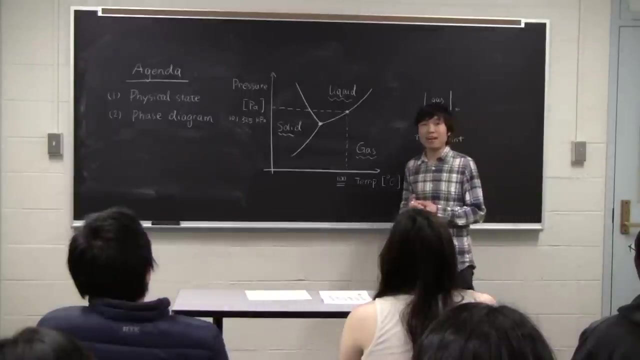 lower than one atmosphere which is less than 1.1 kPa. My question is: is the water going to boil at 100 Celsius, or is it going to boil below or above 100 Celsius? Anyone that volunteer? yes, Okay.